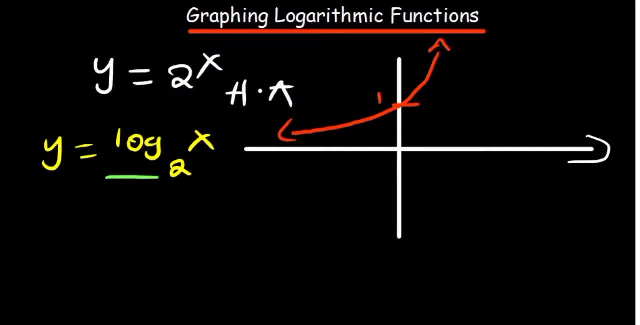 The horizontal asymptote. Okay, That's what we mentioned for the exponentials. So then, as we get to talk about logarithms, we are going to have what we call a vertical asymptote. So it's basically gets to come out like this: Okay, So it can't cut the y axis, And that's. 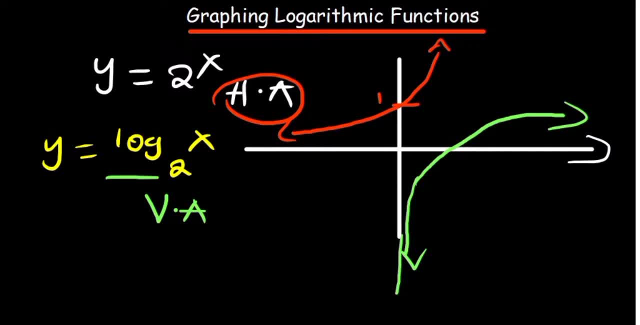 why we are saying it is good What we call a vertical asymptote. Okay, So now there are some of the few things that you have to understand for you to be able to understand. Okay, So we have shown that the y axis is equal to the y curve. How do we get to sketch a logarithm? 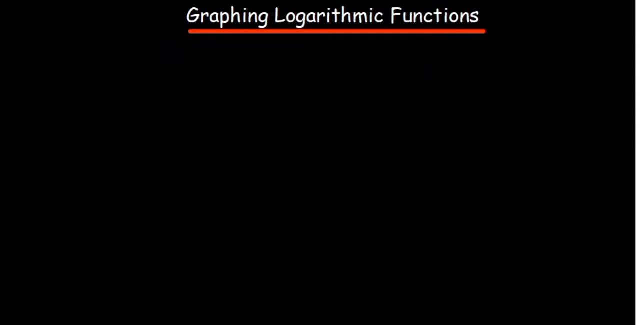 Okay. So, basically, when you have y is equal to the log of x, how do you get to sketch it? So what you're going to be considering is the sin of the log and also the sin of the x. So you ask yourself a question. Okay So, since in that case, what we may have is: 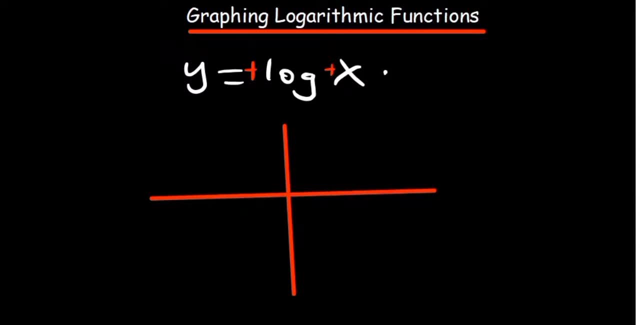 a positive log and a positive x. So in which quadrant are the positive? Where do at the y positive y, Okay, So that's the go toari, and then the e plus. Okay, And the the root. The log of the x is equal to log of x, And we're done. Here is the negative 앉o. 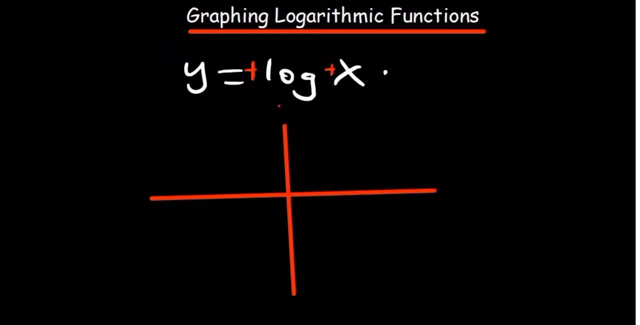 okay, So then we can based this out And we can find addition of two. And what does this positive and also the x positive? it's basically in the first quadrant. so this logarithm is going to basically come out like this: okay, so how about if you get to change the sign? 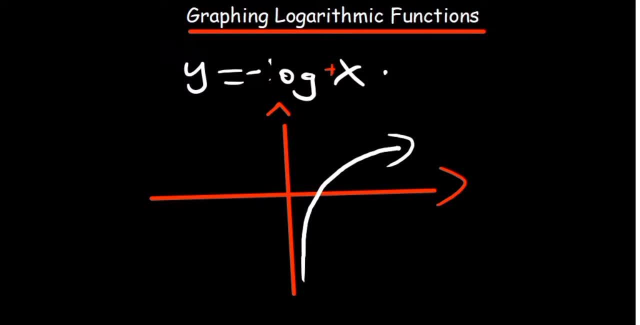 so, if so, if you change the sign of the log, for example, it becomes a negative log. so where is the y negative and where is the x positive? so in that quadrant, that's where you are, the x being positive and your y is basically negative, what quadrant is that? 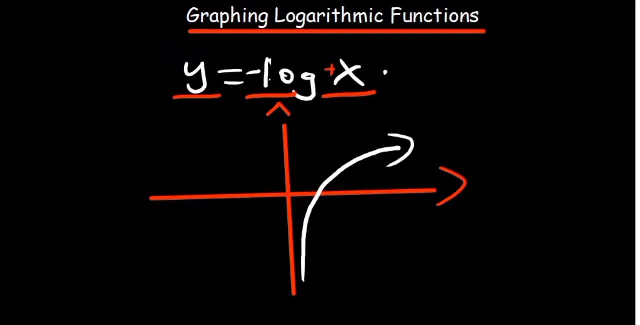 okay, so you can agree with me that in the first quadrant the x-axis is positive, the y-axis is positive, negative and negative. so where do we have the y negative and the x positive? it's basically in the fourth quadrant, so that's where it's going to approach, okay. 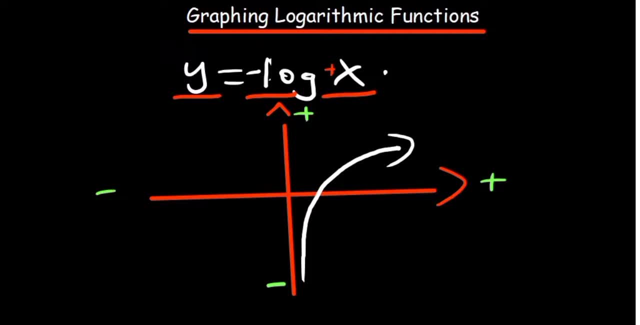 so how is that going to come out, basically? so it's something that is supposed to have been this way, okay, so what we want to maintain is that we want to maintain the fact that the y-axis is going to be our vertical asymptote. okay, so what happens if we change the sign again of um, the x variable? there, let's try to. 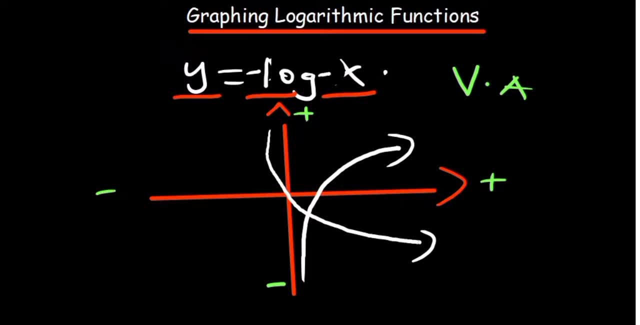 assign this, what we're going to have. let's say, it becomes negative as well, okay. so where do we have both negatives? so it's basically in this quadrant, okay. so what we want is we want the y-axis to be the asymptote, okay, so that's how it's going to come out then, as you. 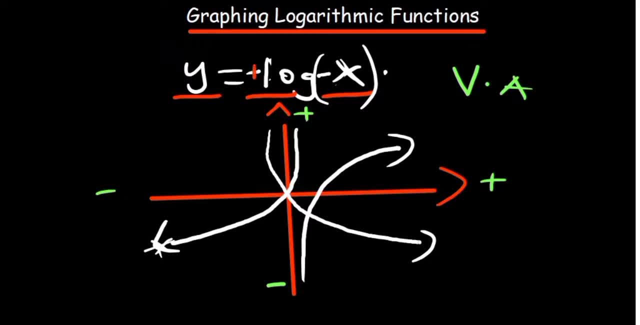 might guess. if the y is positive and the x is negative, it's going to be in the second quadrant, okay? so in such a case, how does it gets to come out? so it's going to be something like this, okay. so these are the important shapes that you have to understand by just looking at the signs. 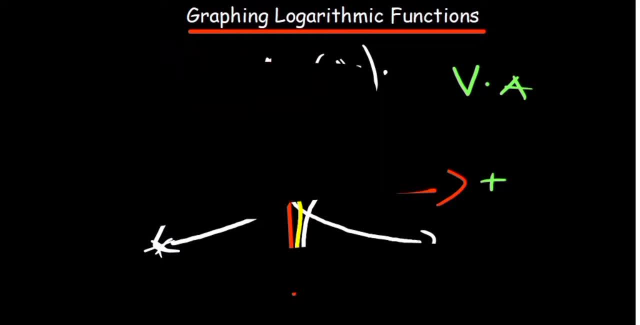 of the logs, you should be able to tell the shape, okay, so i've got a few examples with me that are going to help you more in detail how to go about it. so now let's say you have um, y is equal to log 4, 2 plus 2.. How, basically, can you sketch that graph? Okay, so a few things that we know about logs is. 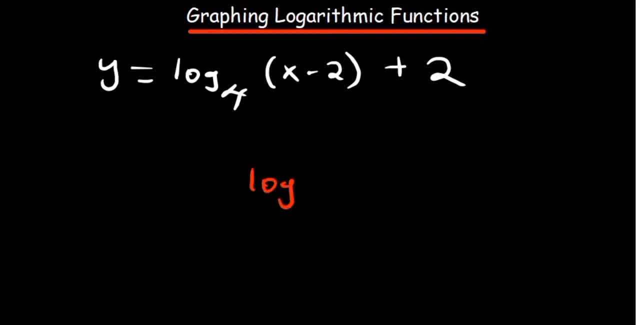 the fact that, log of x and x, this is basically equal to what. So whenever you have got the same base there, you have to know that it's equivalent to a 1.. Okay, so we're going to take advantage of that. So we want to make sure to get to the point where the base is equivalent to what? To the number. 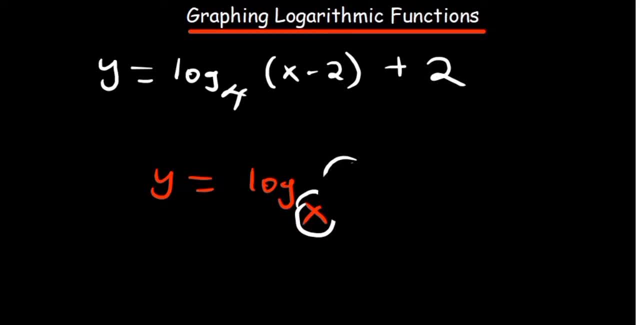 there. Okay, that is one of the things to take part, to take note of. Okay, so that's one. The other thing that we have to know is that whenever you have, y is equal to the log of x. basically we understand that. when you have the log of 0, it's basically what. It's basically undefined, Okay. 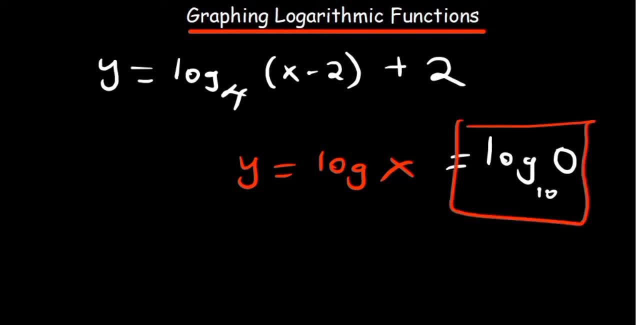 so if you punch that on your calculator, it's basically undefined. So that is basically what helps us to. it gets to give us what The vertical asymptote. So whenever you have the value of x there being equivalent to a 0, then that will. 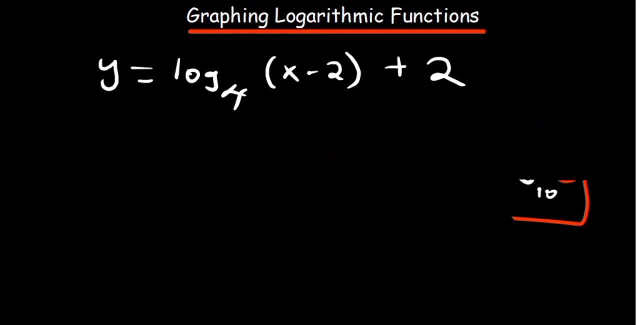 be your vertical asymptote. So we've talked about the vertical asymptote. We've also talked about the point where this is equivalent to what you have in brackets there. Okay, what else is really important? What else is going to help us? So the other thing that can help us is a fact: when what? 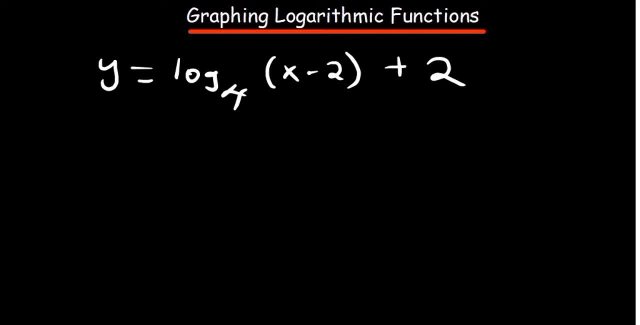 you have in the brackets is basically equivalent to a 1.. So what else is going to help us? So the part of 1.. Because what we understand is that whenever we have any log with the 1, there it's basically going to be- I can write this in another form- to say to the power: 0,, which is basically: 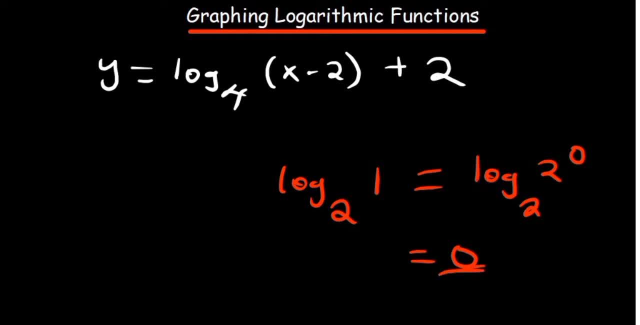 going to give us a 0, yeah, So in case you don't understand what that is, check out our video on the basic logarithms. So we know the three things that are very important, that can assist us when sketching. So let's come up with our table values. So we have x and y. The first thing that we've said is we need to make sure that every base randomness DONT Vinовать Das 2, das sind E without 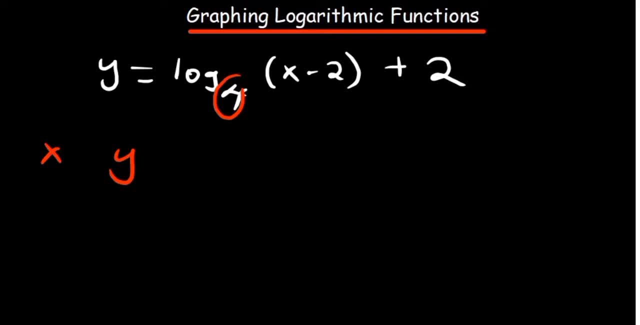 sure that the base is the same, right, because when we have the same base, we are saying this is equal to a 1, so let's try to get what's in the brackets here. what we have is x minus 2. so when x minus 2, 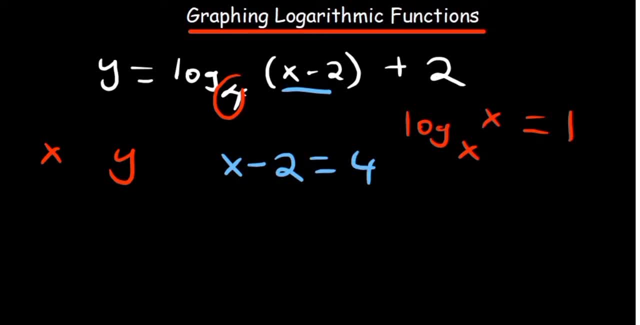 we want it to be equal to 4, we equate it to 4. so this is going to be true when x is basically 2 plus 4, which is a 6. so when our value of x is equal to 6, our y is going to be 4. so we've come. 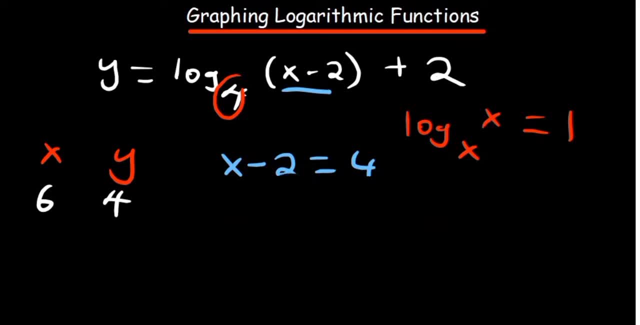 up with a first point here. the other point that we are mentioning is we want to make sure that what's in the brackets is equal to 1, because whatever base you're going to have, provided it's 1 there, it's basically going to be a 0, because we'll make that to be a 4 to power 0. 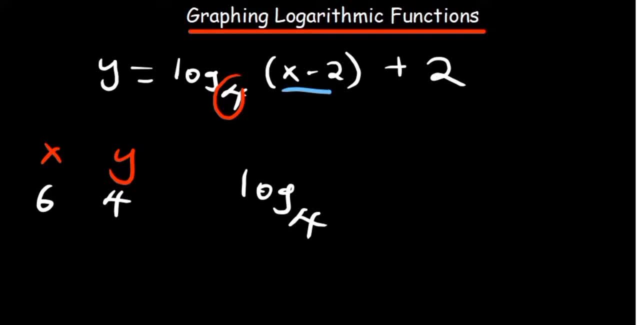 okay, so in this case, what we have in the brackets, what we have in the brackets is x minus 2. so equate x minus 2, equal to being a 1. so you're going to find that x is basically going to be a 3. 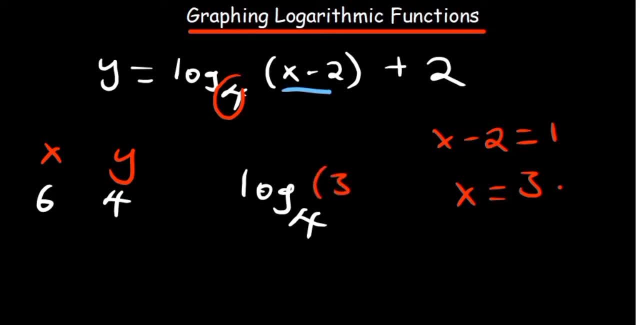 okay, so that when you put 3 minus 2, what you're going to have is what is a 1, so you have a 4 power. what the power? the power: 0 when x is equal to 3. so at that point, what value are we going to? 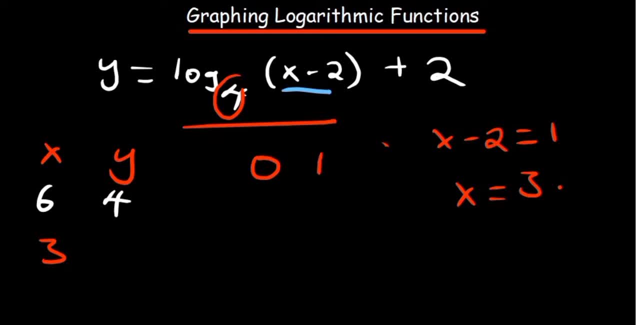 get. so this part is going to be equal to a 0 plus a 2, which is going to be a 2 there. what else do we have to put into consideration? so i have to put into consideration what we're calling the vertical asymptote, the point where we don't expect it to cut. 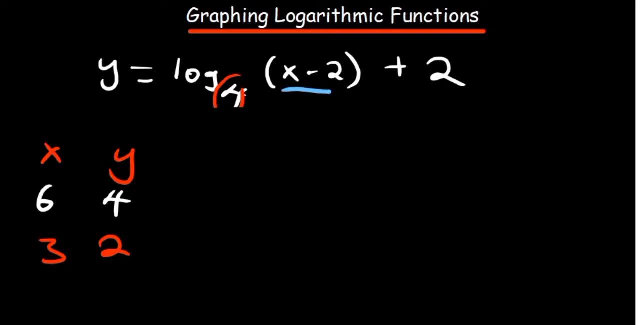 the y, the certain y axis. so we are saying that gets to happen when basically, your value of, let's say your value of x square is equal to 0. it is undefined, so let's try it out. so want x minus 2 to be equal to 0. this can happen when x is equal to what? when x is basically equal to a 2. 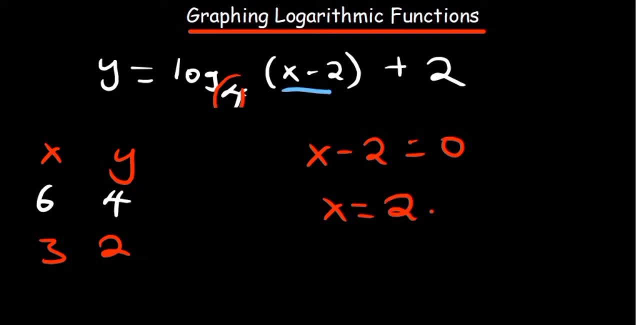 okay, so our vertical asymptote is when x is equal to 2. that is our vertical asymptote. so with this information we're able to sketch our logarithm there. let's try to sketch it, okay. so what do we have? so we have- at least we have- x, so the smallest value that we have so far. 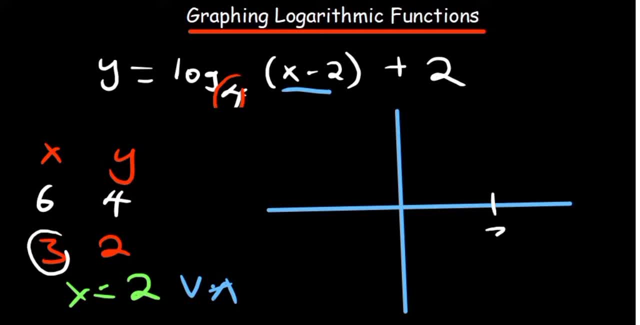 is when x is equal to 3. so when x is equal to 3, we have x square is equal to 3, your y is equal to what? Your y is equal to 2.. Then we also know that when x is equal to 2, that is our vertical asymptote. So we can show it. We don't want it to cut. 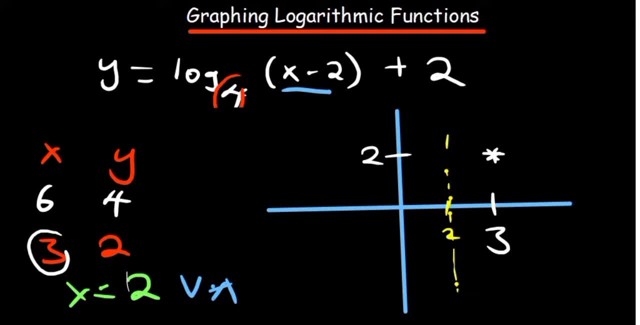 that line. Then the other thing that we know is that when x is equal to 6, our y is equal to 4.. Somewhere there 4, somewhere there. So we now understand the shape. So it's basically going to be something like this: It shouldn't cut y, it's equal to 2.. So what is the shape? 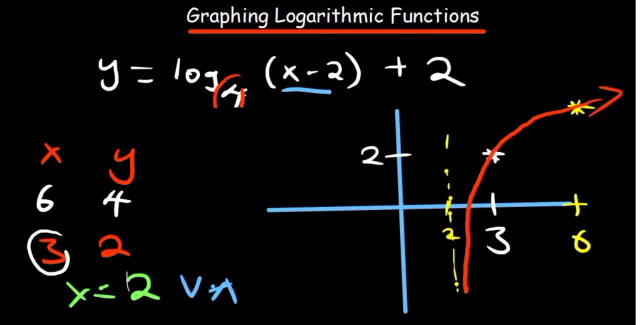 of our logarithm there. So, basically, the point that we're trying to make is that in this case, our vertical asymptote is 2 and we understand. by looking at the sign of the y-axis, we're able to see that it's supposed to be that way. That's the shape. Okay, let's try. 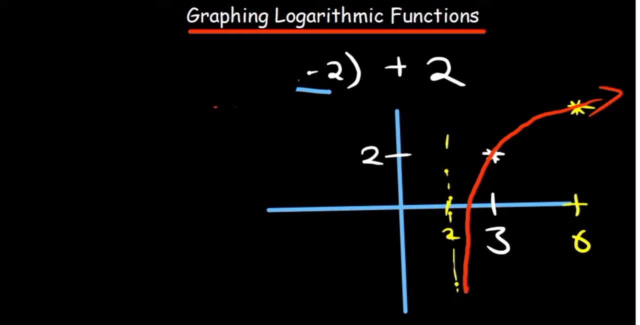 to look at another example, It gets to understand more how to go about it. Now let's say in this example, let's say our y is basically equal to log 3, x plus 1.. So there are just a few things that we've talked about. We've said that we need to make sure that what's 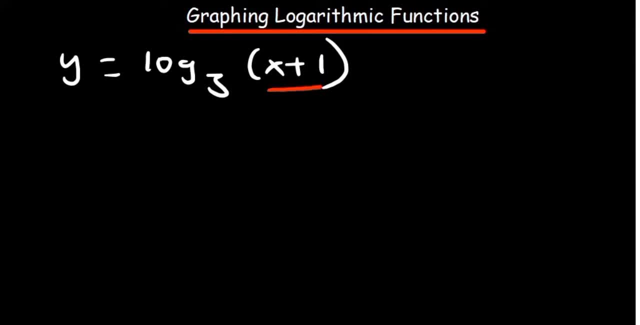 in the brackets is basically equivalent to the base. Okay, Because we understand that whenever you have the same base with a value there, that is equal to a 1. So we want to use that property to help us. So let's try to equate. 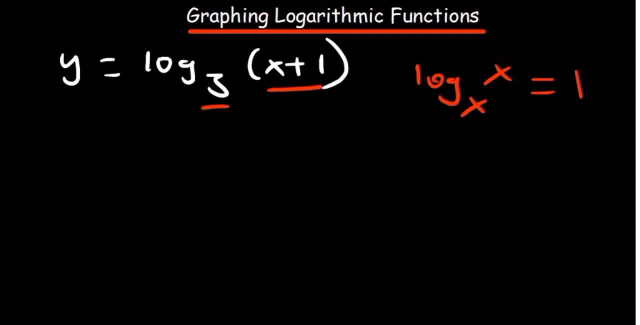 what's in the brackets- to be equal to a 3, because that's the base that we have in this case. So what is going to be true when, basically, our value of x is equal to what It's equal to 2.. Okay, So we can come up with that. So we're saying, when x is equal to 2, our y is. 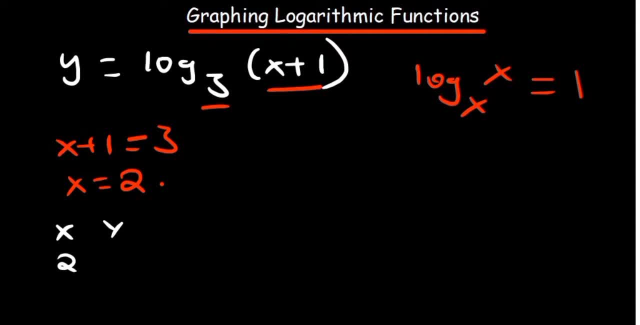 going to be what Our y is going to be basically equal to a 1.. So in this case we don't have anything being added, So it will just be a 1 itself. So that is going to give us a 1.. Then another: 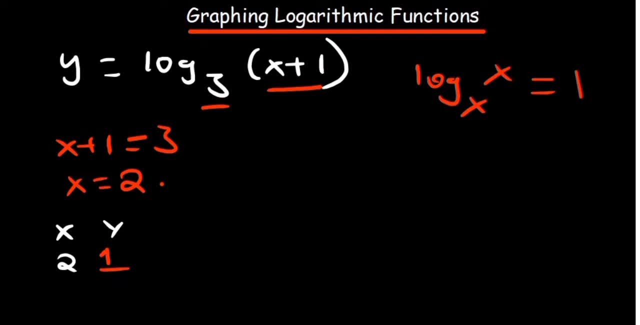 property that we're trying to take advantage of is: we don't want this to be equal to 0, because when it's equal to 0, it means that it's undefined. So x plus 1, when is it equal to 0?? So it gets to be equal to 0 when x is equal to negative 1.. So when x is equal to 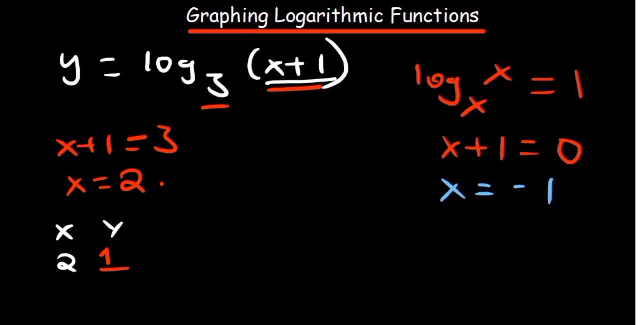 0,. what is our vertical asymptote? So x is equal to negative. 1 is our vertical asymptote. Then, another value that is very important to come up with is when what's in the brackets is equal to a 1, because whenever it is equal to 1, what we expect is that when you have 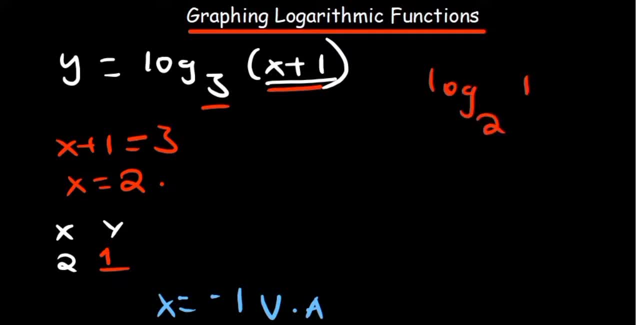 any base with a 1 there. what it means is you can express that to the base raised to the power of 0. And if you take it the other side, what you're going to have is a 0 as your solution. Okay, so in this case, the only value of x that can give us a 1 is 0, because when you 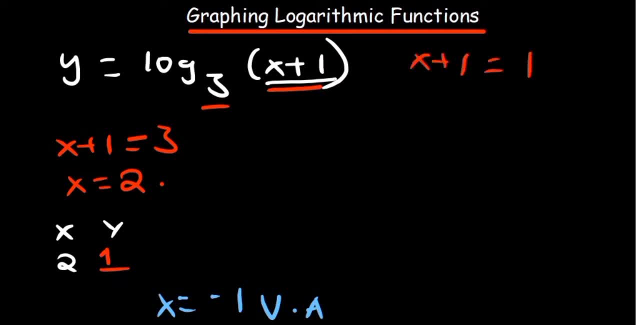 have x plus 1, this is only going to be equal to a 1 when our x is equal to a 0. So, when our x is equal to 0, what are we going to have? So, when our x is equal to 0,, what we're? 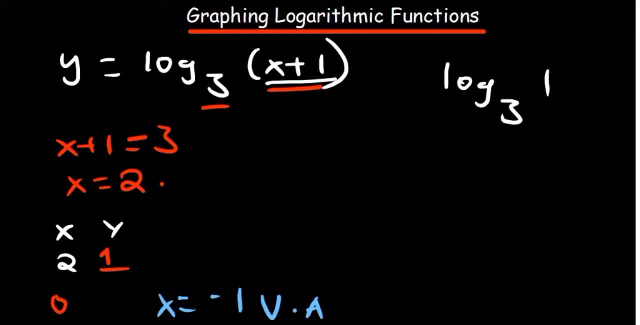 going to have is log 3, 1.. Okay, So at that point it's going to be log 3, the power of 0, which is just going to be a 0.. Okay, so it's basically 0, 0. 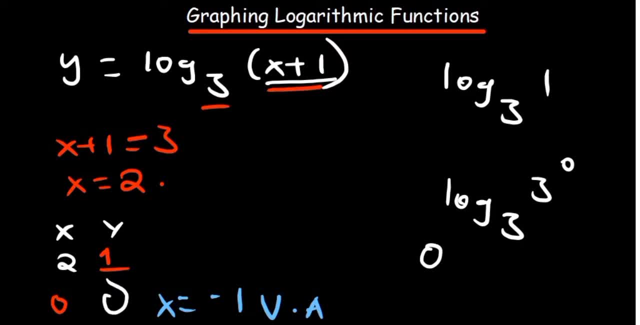 That's what we have in this case. So we have our vertical asymptotes. We also have the cardinal 3, 2 coordinates to help us sketch it out. Okay, let's sketch it now. So where is our vertical asymptote? 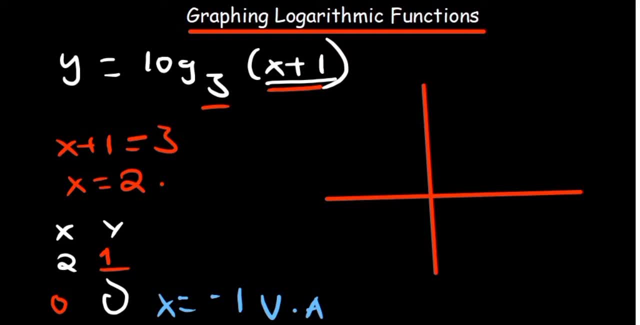 So our vertical asymptote is basically: x is equal to negative 1 at this point. okay, So we have our vertical asymptote. Then we also have a point we expect it to cut at: x is equal to 0, 0, that point there. 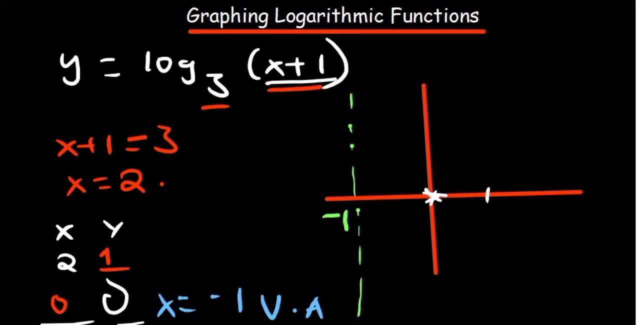 And the other point that we have is 2, 1.. So 2, 1, somewhere there. okay, So, basically, we're able to see the shape. Okay, Okay, Okay, Okay, Okay. So that's what we have there. 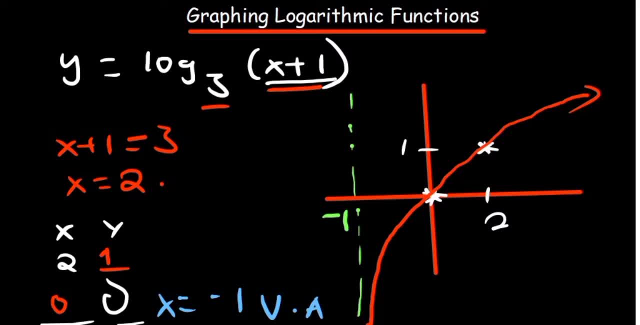 And in such a case, when they ask you to sketch such a graph and they ask you for the domain, so for the domain, what they're asking for is the values of x that can define the function, And we know that negative 1 is going to make it to be undefined and we can't pass going. 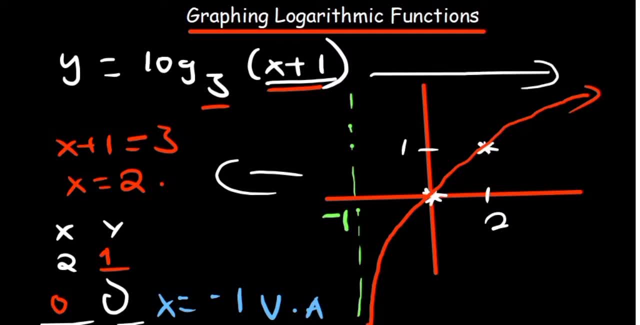 this side, So we are only limited going to the right-hand side. So in this case, what we can say is: for our domain, for our values of x, the minimum we have is negative 1. one, but negative one is not included, and thus we have to use a curved bracket. so 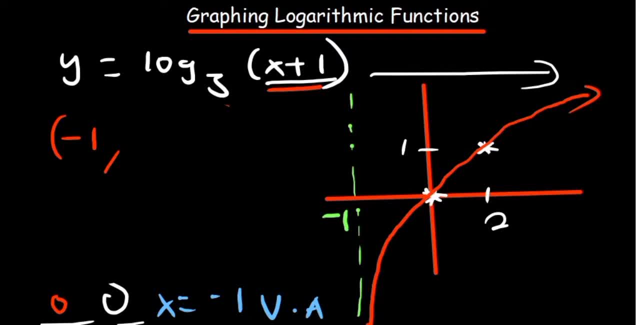 it's all the way from negative one up to positive infinity, because it's not ending. this side, that is for our domain. okay, then, for our range. our range gets to define the values of y. so for the values of y, we are going down there. it's. 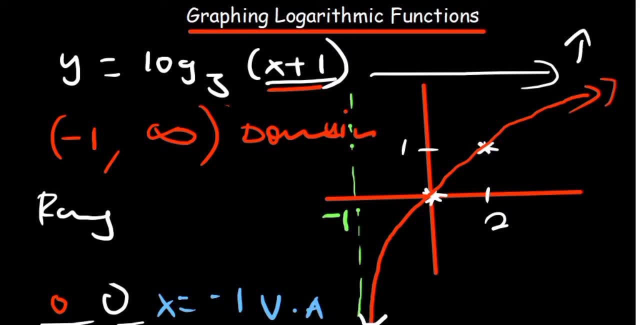 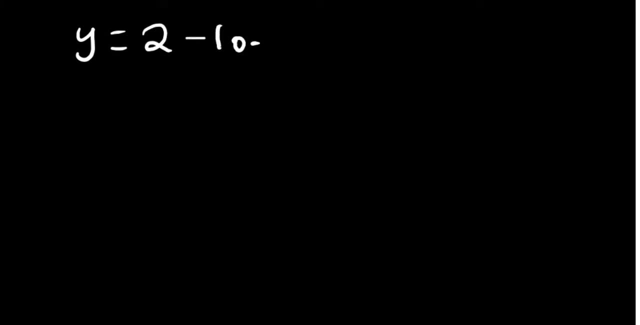 unlimited. we're also going up there, so it's basically from negative infinity to positive infinity as our range in such a case. okay, let's look at one more example, a very unique form, where you start with something, then you subtract the log. okay, how is this one different? how do you get to sketch it? okay, so 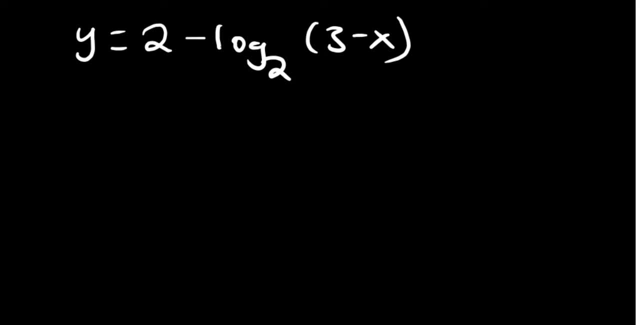 taking note of our properties. what you're saying is that let's come up with our values of x and y. we want this to vote to think of on a point where the bases are equal, right with what is in the brackets. so in this case we have a base of 2, so 3 minus x. when is it going to be? 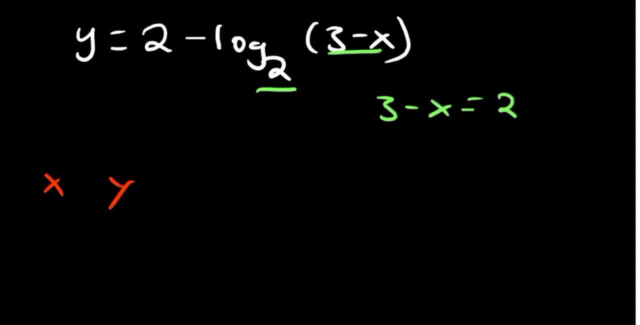 equal to 2, so it's basically going to be equal to 2. when you have 3 minus 2 is equal to x. so when x is equal to 1, so the moment x is equal to 1, what are you going to have? so, when you plug in x to be equal to 1, what you're going to have? 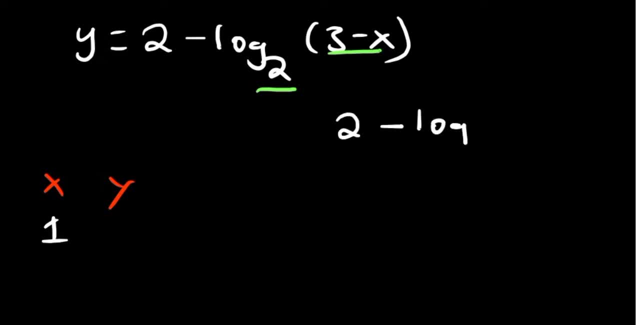 is 2 minus log 2. so in the brackets where if you put a 1 there it's going to be a 2, so you have log 2, 2 and so on, so we have 2. so whenever I've got the same base and the value of that is: 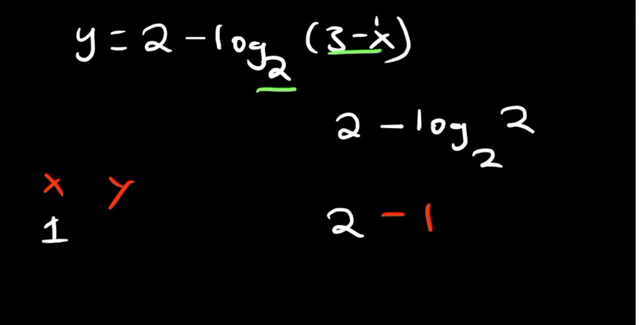 basically a 1. so we have 2 minus 1, which is going to give us a 1 there. another property that we are taking note of is when what's in the brackets is equal to 1. so when do we expect to be 3 minus 6 to be equal to 1? so basically, 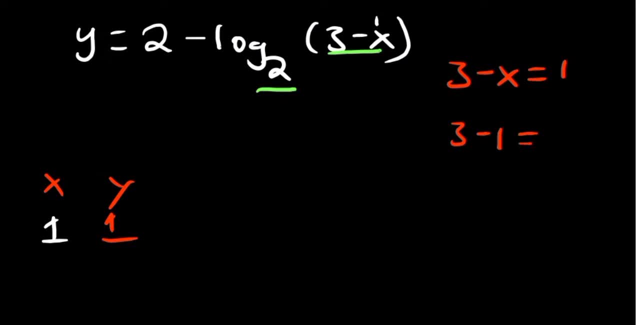 what we are going to have is: 3 minus 1 is equal to x. so when x is equal to 2, and so when x is equal to 2, what we expect is that in the brackets, what we're going to have is a 1, so we're going to have our y being equal to 2 minus log 2, then a 1. 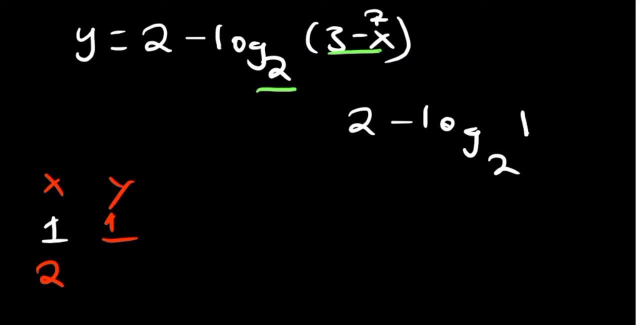 there, because if you put in a 2 there it will be a 1. so the 2, the one there, is the same as the base 2 raised to the power 0. okay, so this part is going to be equal to 0 from the logs. okay, so our logs still teaches us to say: 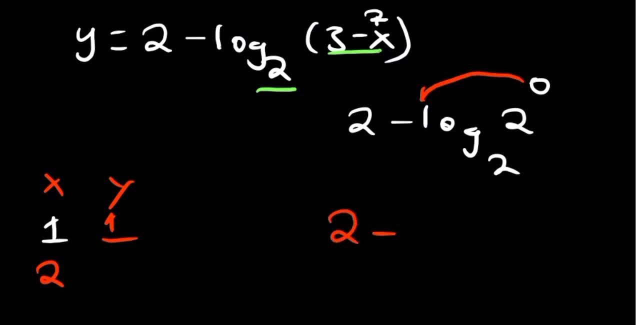 that that can come this way. so we have 2 minus 0. then log 2, 2. so log whenever you have the same things there it's a 1, so you just have basically have a 2. so two properties have been used: one where the brackets are equal to 1 and also when 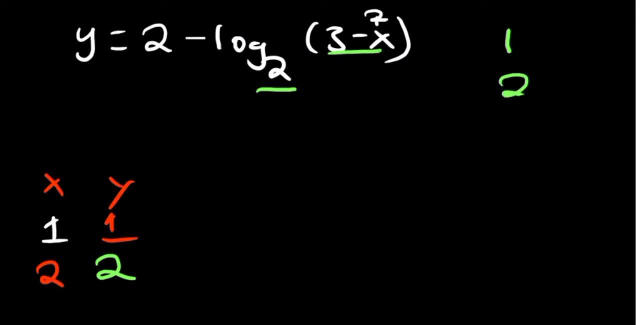 they are equal to the base, in this case, which is a 2. so we've come up with coordinates here. then another thing which helps us to determine the vertical asymptotes is we are saying: when do we expect what is in the brackets to be equal to a 0? so 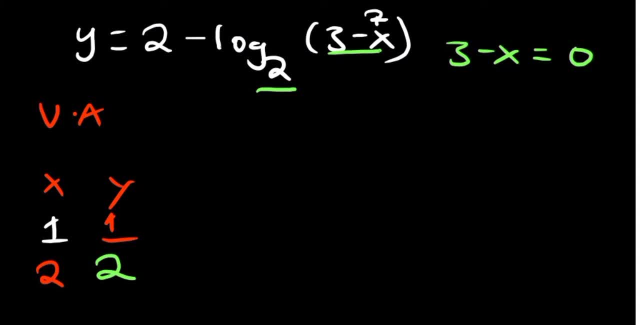 3 minus x, can is only can only be equal to 0 in our x is equal to what? 3? so that is our vertical asymptote. so okay, so with this information we should be able to sketch it out. okay, let's try to come up with our graph. we see, though it's. 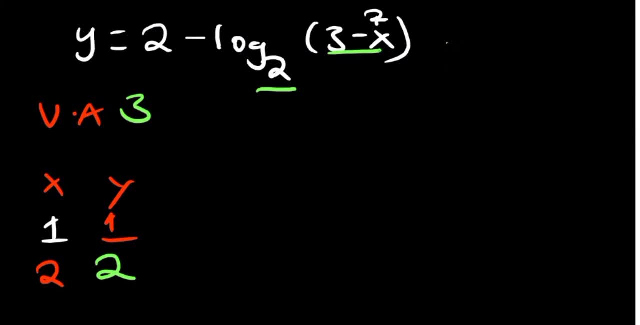 going to come out? how do you expect it to come out? so that's what we have, okay, so our value of first coordinate there is 1 comma 1 somewhere there. then our other value is 2 comma 2 somewhere there. okay, so for vertical asymptote, what? 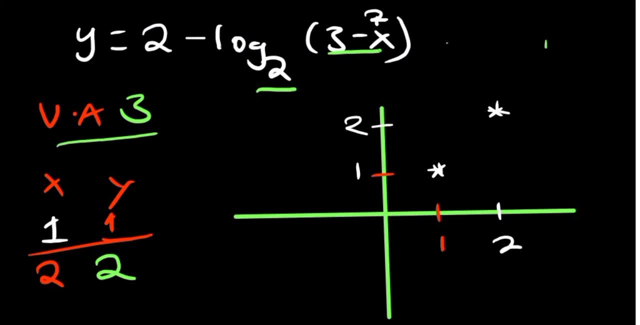 we have. we have, y is equal to what our x is equal to 3. sorry, somewhere there, let me use a different color so that it looks better. you, I'm going to use a different color, so that's what we are going to be able to do. so what is our vertical asymptote? so how is the graph going to come out? so 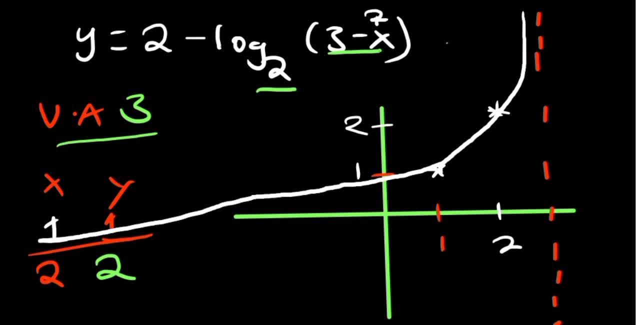 so it's going to come out like that. so eventually it's going to cut the x-axis and going to get down there, but it's going to take some time, but as is how the shape comes out for that log. okay, so in this case, if I ask you to find the